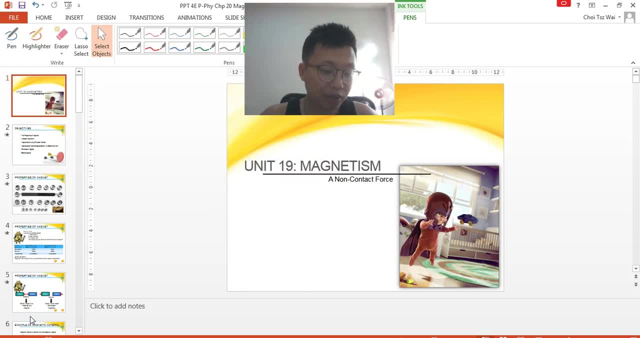 do very well in this chapter. okay, so what this video will do is that I'm going to go through with you some main concepts in this chapter. for example, we are going to talk about how magnetism arises, and to do that, I have to introduce a new concept to you, and it is called domains and, by the way, there will 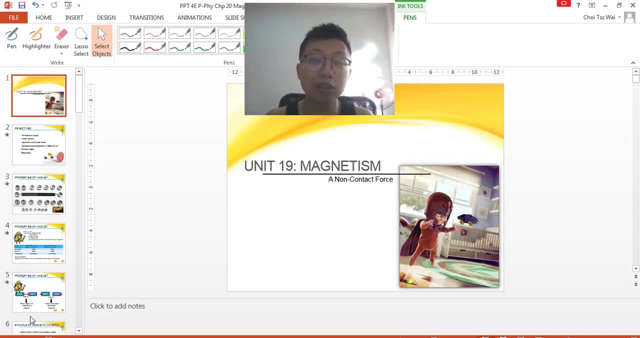 be no notes, so you need to take down your notes, and I think your teacher is going to check your notes to confirm that you have watched this video and that you have picked out the key concepts that that we will be talking about later. okay, then, after that, I have to introduce you to a new rule that has something to do with 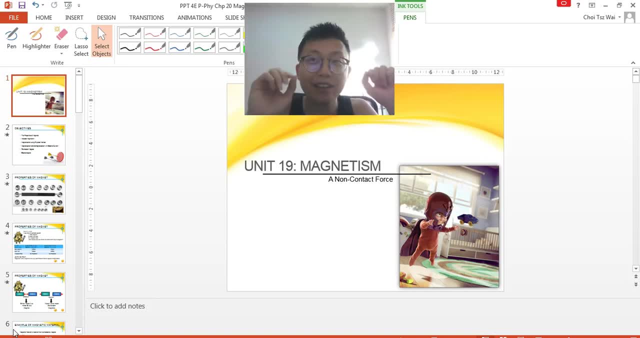 your hands. so for the next chapter, you will be hearing things like right hand grip rule and you have to use your right hand to to do that rule, and you have your Flemish left hand rule and you will have your Flemish right hand rule. so for 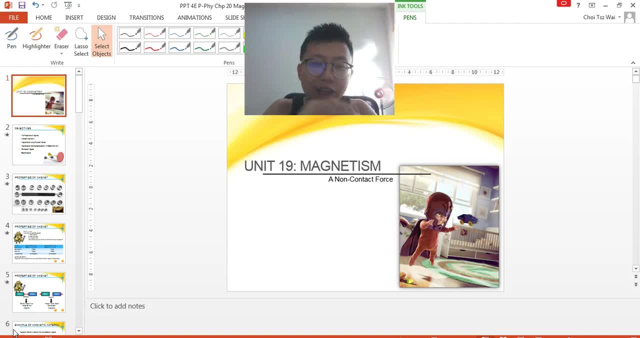 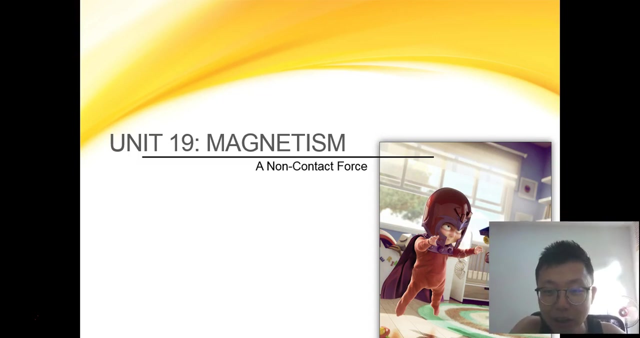 those in Chinese called 左右部分, or you cannot determine which is your right and the left hand. it is time for you to find a way to differentiate right and left. okay, so, without further ado, let's begin our chapter, and I will minimize this thing and maximize my very cute magneto baby. okay, magnetism. so 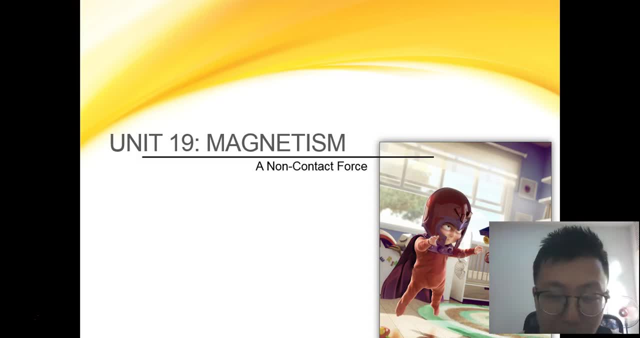 before I go on and discuss about magnetism. do you know who invented the magnet? any idea? actually it's a trick question. no one invented the magnet. actually, the magnet was found. so legend has it that the good man invented the magnet. and the magnet was found. so legend has it that the 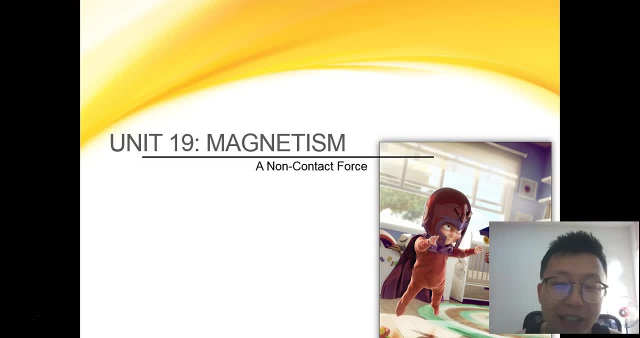 Greek has is the one that has discovered the magnet, and that the story goes that there's this farmer who was walking along the road one day and his shoe nail. I do not know what is a shoe nail, but you can google it, so I assume that it must be a metal part of his shoe get stuck onto one of the 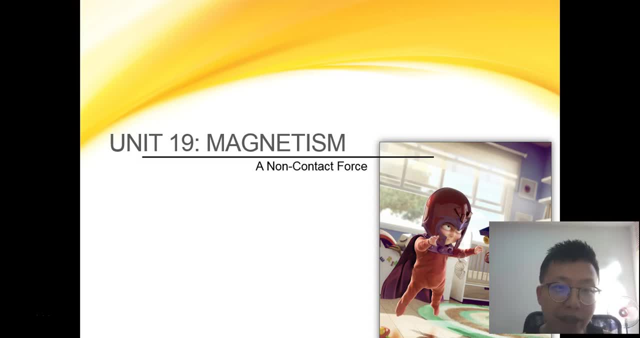 stones. so apparently this stone has some magnetic material embedded in it and because of that, the magnet started to get attracted to the iron nail on the shoe, and so they discover this mineral that would be attracted to iron or steel, and they decided to name this material magnet, and legend also said that it is the Viking who who? 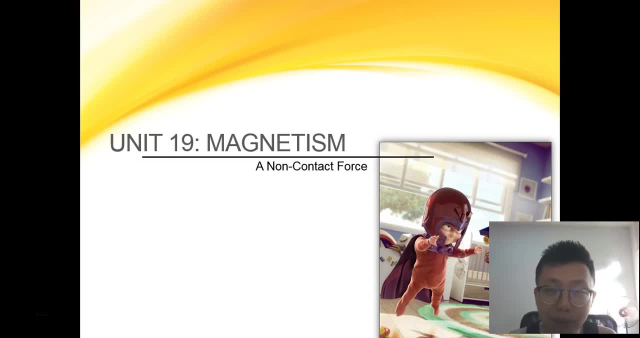 because they have discovered the magnet and use it as a guiding compass that England and invaded England. but if we rely on historical record, it is actually the Chinese who first make use of the magnet as, oh as a tool to, to navigate. so, fun fact: do you know how a magnet, how the, how do, how the, how, how a compass? 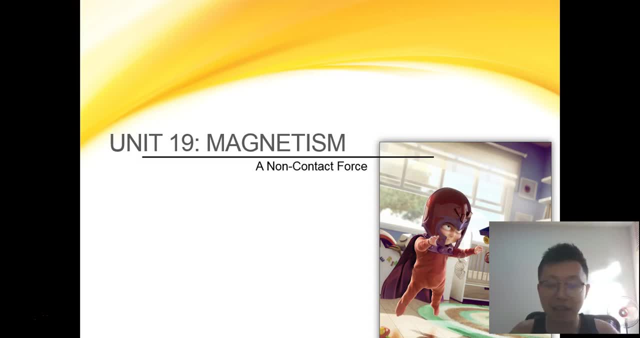 work. yeah, yeah, sorry, I always get it when I'm teaching, so anyway, this is the fun fact. so what happen is? I needed to look at the slide. basically, a compass is actually a magnet, so and of course, I expect you to know that the the rule of magnetism, similar to 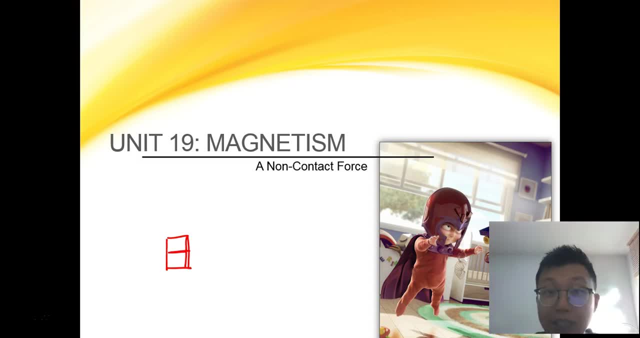 the rule of electrostatic. the rule of electrostatic is what it says like: attract according to the scale. you will attract electricity in your time. the light pole will attract electricity in your time. the light pole repel and light pole attract right. so similarly, the rule of magnetism is that light 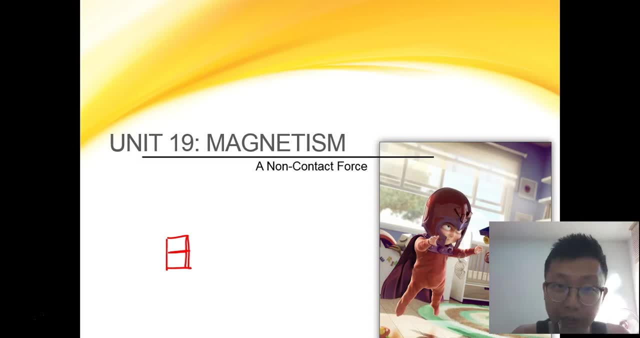 pole will repel and, unlike pole will attract. so what happened is that your compass is actually a magnet. so your compass will interact with the earth magnetic field and it will only point at a fixed direction. so, uh, what i'm drawn here is actually a compass. this circle is the housing. 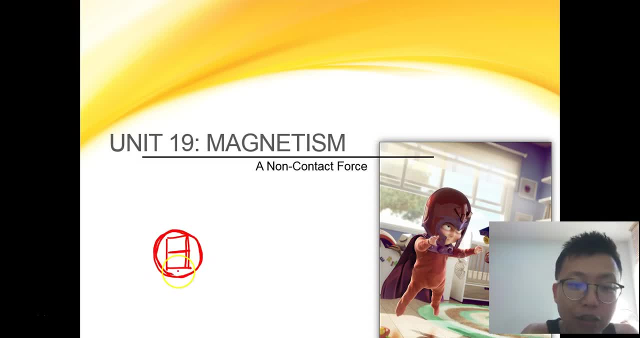 of the compass and the needle of the compass is actually a magnet. so, uh, we decided that to name this your geographic north. that means whenever this, this compass needle, is pointing, it is the north, and whenever the other end is pointing is our self. so we decided to name it like this. 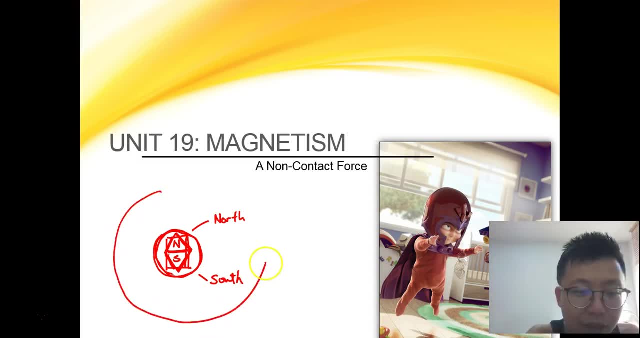 but if you think about it, so this bigger circle that i'm drawing is the earth, the planet earth. so if you are saying that this compass is pointing at north and you know that, unlike pole attract, so if this is north, then what is the magnetic pole on top of the earth? if 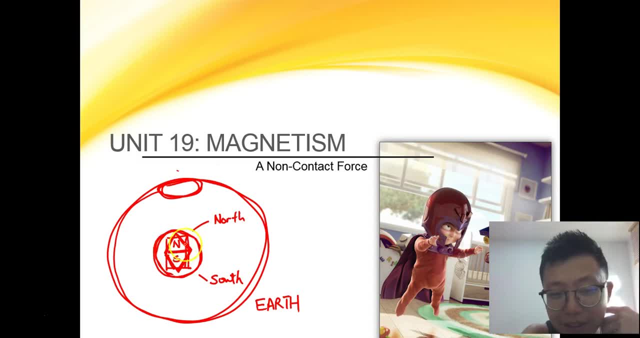 if this is north, then what is it attracted to? the magnetic self, right? so actually, our earth, our geographic north, is actually our magnetic self. so, even though we call the the top half of our earth, the north part, or we call it the north pole, because this is how we define, 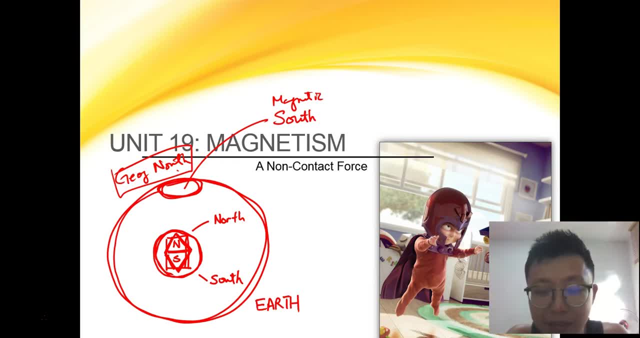 it geographically, but in terms of magnetism it is actually the magnetic self. so actually the bottom of the earth, which is our geographic self, is actually our magnetic north. okay, so this is a bit of fun fact. so, uh, just now i have mentioned that uh magnet is actually found and it is not uh being invented. that means not. 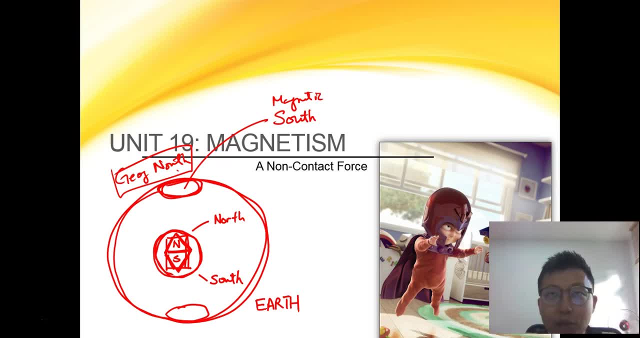 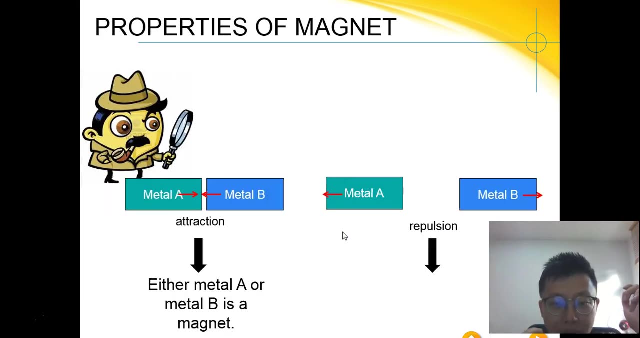 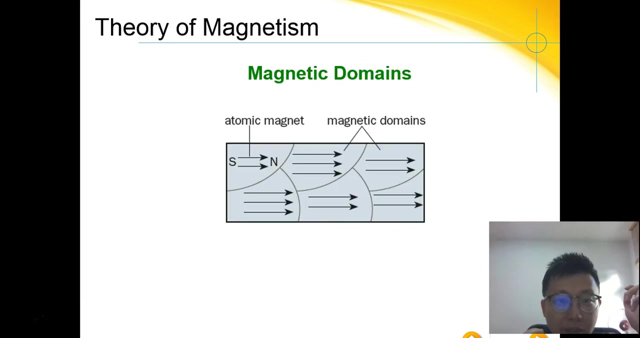 someone, uh tried to make it, okay, it was found. and then, uh, it was actually found deep under, uh the earth. so what happened is that? um, to explain magnetism, we have to talk about this thing called uh domain, so i'm going to skip this. okay, in this science model, right, we are imagining that. 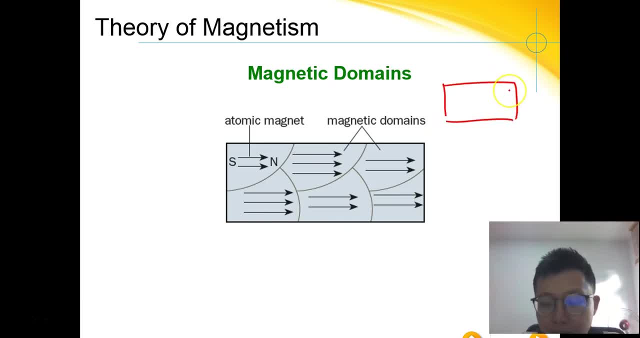 when we have a piece of material. instead of using the kinetic model of matter, we only learn two model. the first model that you learn is kinetic model of matter and the second model is kinetic model of matter and we learn that, using that model, a solid is makeup of particles that are in fixed 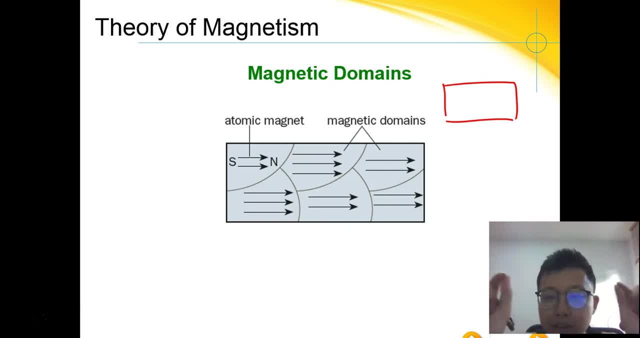 position, vibrating about their fixed position and there's very little gap in between them, and so on and so forth. but for this model that we are going to use, we imagine that this rod is actually makeup of domains, and these domains is actually. how do i, how do i know that? why is it that i call this a domain? because we imagine that all 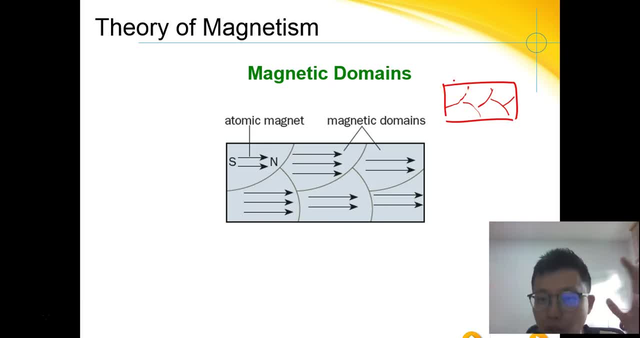 these particles are being grouped together as a domain, and why do we group them together is because that these particles are all pointing at a certain random direction for a non-magnetic material. so basically, you can imagine that this domain are tiny magnets and when i draw an arrow like 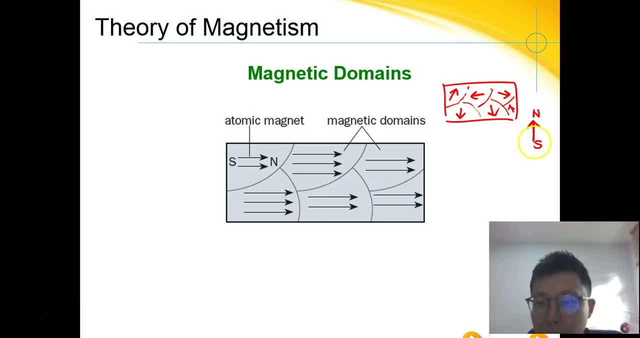 this. it actually represents north pole here and south pole here. so actually all solid, all materials are having this domain. but why is it that they are not magnetic? it's because these domains are not aligned. they are all randomly scattered. so let's say: i have a north here. it is being 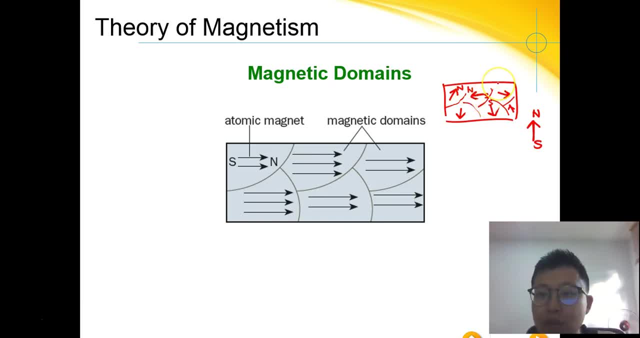 neutralized by this north and then this self is neutralizing this self. so, because of the randomness of the domains and the direction of the domains, i can see that the domains are all pointing at random direction. there is no net direction, unlike this diagram that i am showing you. 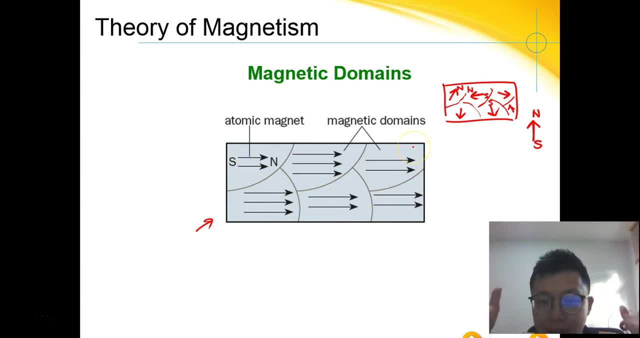 so can you look at this diagram and you can see that the domains are all pointing at a single direction, meaning that the north here will actually be be aligning this domain, and then you can see that all your north is now pointing the right. so what happened is that when you zoom out- and you will 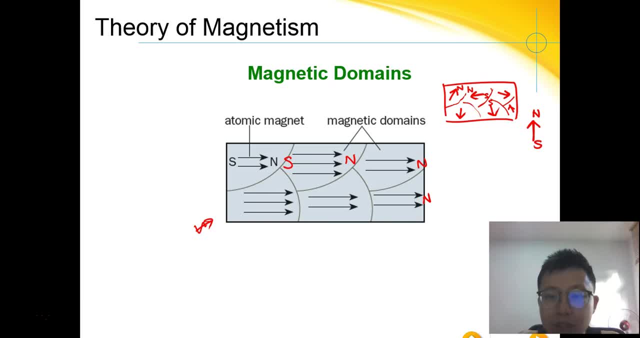 this material as a whole, then you will have a net north pole on the right and you have a net south pole on the left. so in physics- i summarize- we imagine that a material is makeup of domain. so for a non, so for a material that has not been magnetized, its domain are all pointing at different. 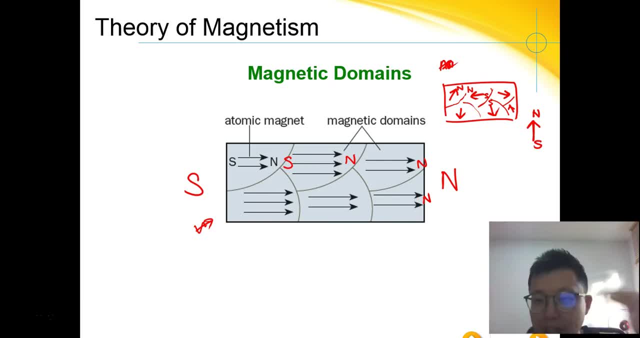 direction, and because they are all pointing at the same direction, they are all pointing at the same a different direction. there is no net direction. the domains are not aligned. so because of that there is no net magnetic effect and because of that the material is not magnetic. but if we somehow 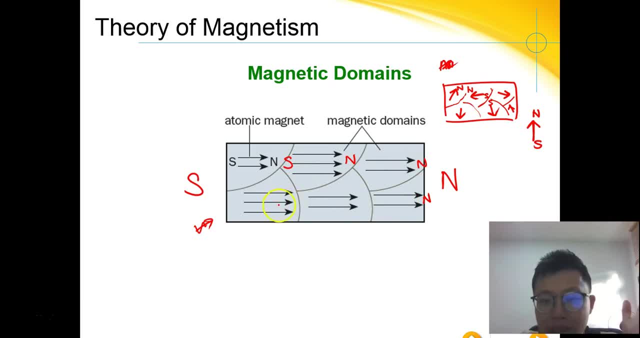 manage to align this domain in one single direction, then this material would become magnetic. okay, so you may ask me, teacher, so, uh, so far you have been. you have told me that, okay, materials, natural materials, will have his domain pointing at all the different direction and because of that, uh, 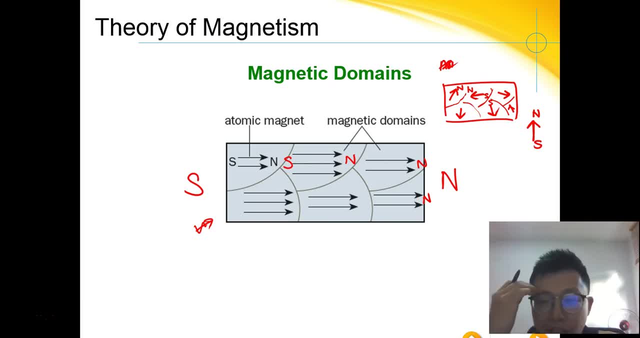 natural material does not, is not showing any magnetic property. then why is it that you say that in asian time, magnet is being discovered? how can they discover something that is not naturally occurring? remember, uh, the story that i told you about how the greek farmer discovered that this stone will get stuck to his uh shoe- iron shoe nail. so what happened is that when 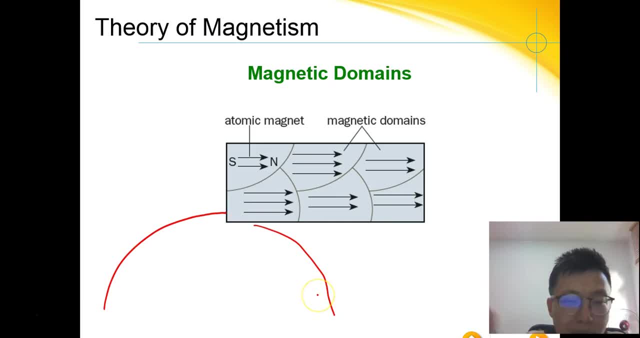 let's say now this is half of the earth. so what happened is that when, when you have iron or some material deep under the earth, this material are actually under great pressure because of the many the thick layer of soil above it and also because it is very near to the core of the earth, so the core of the earth is very hot. so, basically, when 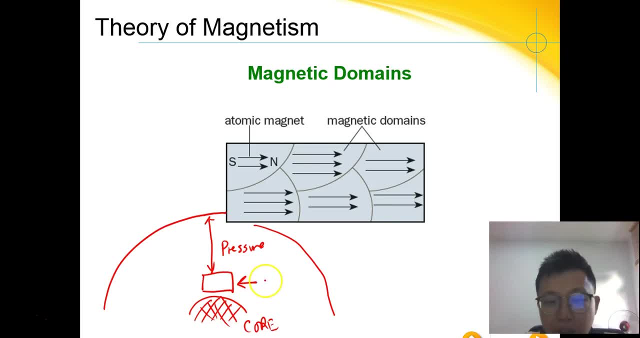 when you have minerals deep under the earth, it is actually under high pressure and high temperature. so when you have high pressure and high temperature, that means the particles in this material, these minerals, are actually very energetic, it has a lot of energy and because the earth has its own natural 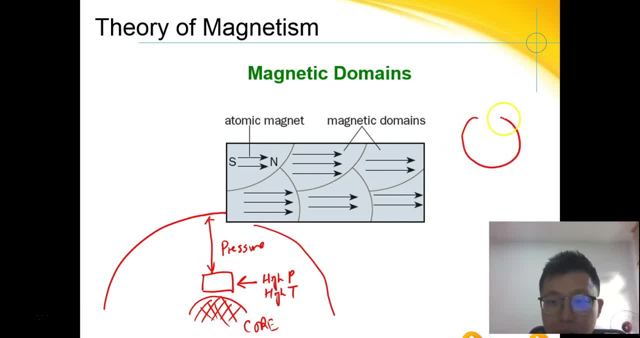 magnetic field. so the earth has its own magnetic field, right? i'm sure you have seen some nasa diagram that shows something like that. and then this is the earth magnetic field. that is like 3d and it's like a butterfly, things like that. so what happened is that when you have a mineral that is deep, 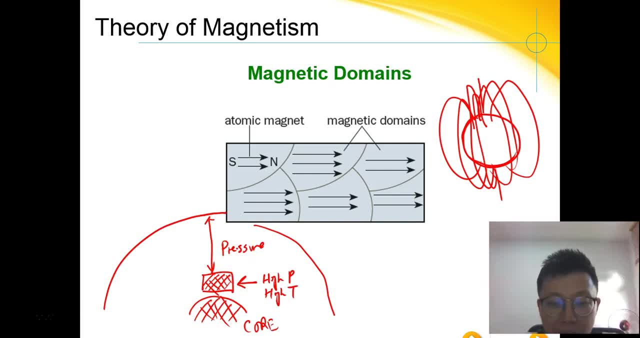 under the earth and it is under high pressure and high temperature. these particles are very energized, meaning that they are very mobile and because of that, and and because of that, and that you have a magnetic field from the earth, the magnetic field from the earth will start to slowly align the domains in a singular direction. so let's say: 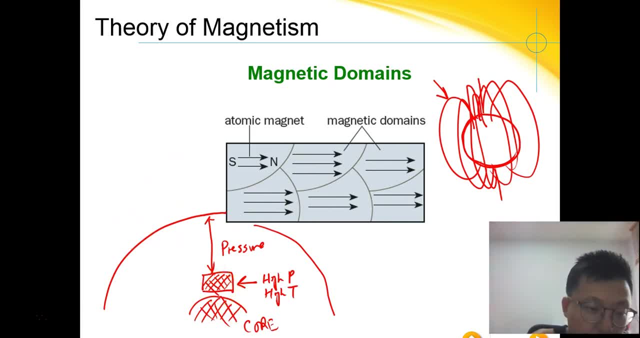 this is, this is the earth, and i have a magnetic field that go this way, this way. so what happened to this mineral? is that? because it is, because its particles are very highly energized. okay, let's say at the beginning: the domain of this material is all. 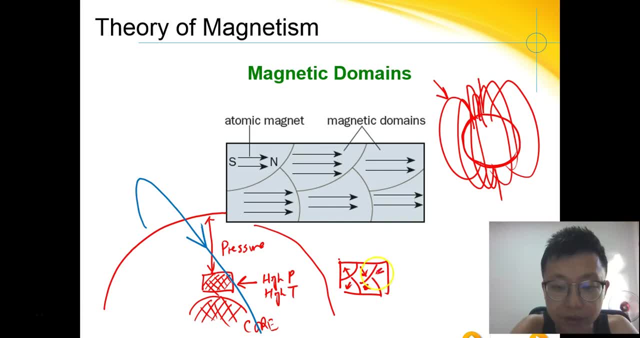 haywire, all pointing at different direction. okay, but because of this magnetic field. so there's a magnetic field from the earth which is naturally occurring, going by this way, because the domain are very energized, so they can move around slowly. okay, although it's not like immediately. 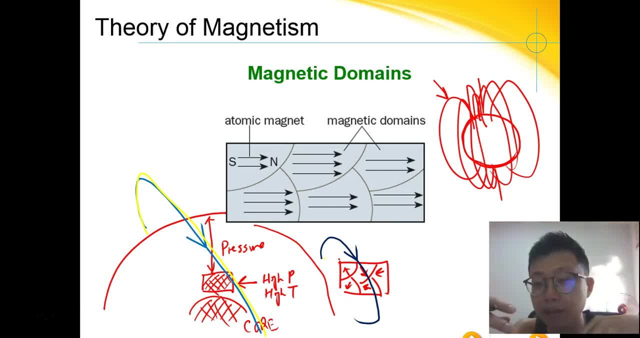 change direction, but because it is very deep under the earth so it has a lot of time, it has temperature and it have an external magnetic field. so this external magnetic field is like a person, it's like a teacher shouting at a group of set one student. so the set one students. before the teacher come they are all. 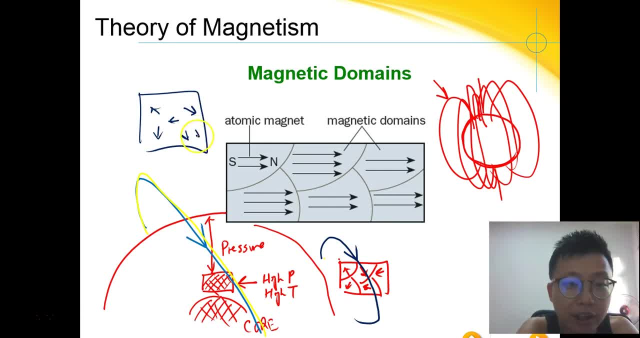 looking at different direction. right, so these set one students are like your domain in a, in a normal mineral, they're all looking at different direction. but once you have an external magnetic field, who come here and you start shouting: hey, so what will happen? your student will start to, slowly but surely. 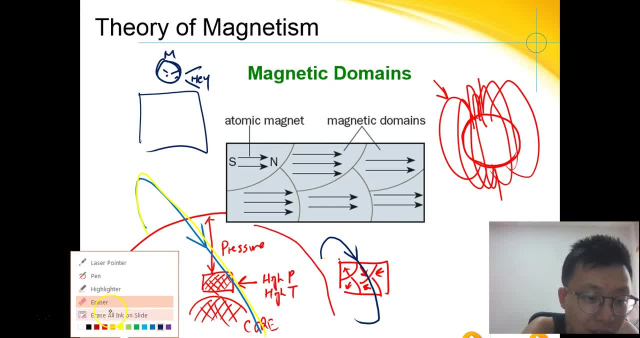 although some of them, like you guys, will not listen, but they will surely eventually turn and then face the teacher right, and then you will have a group of student now facing in a singular direction. so, similarly, this external magnetic field will have this effect of slowly turning all this. 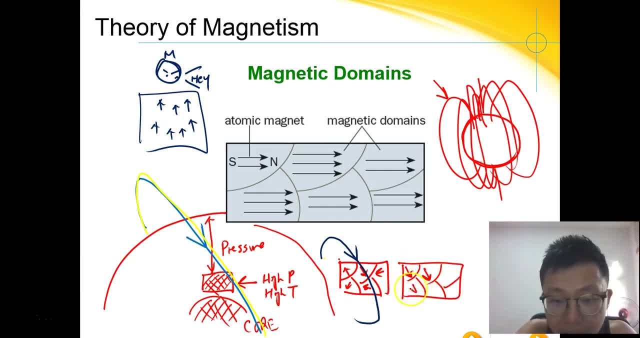 dipole and then aligning them in one single direction. and when this happens, when this condition is being fulfilled, then you will have a magnet that has north here and south here. so that's how magnet form and you need to understand the scientific model that we use to explain how magnetism arises. basically, it is the alignment of domain. 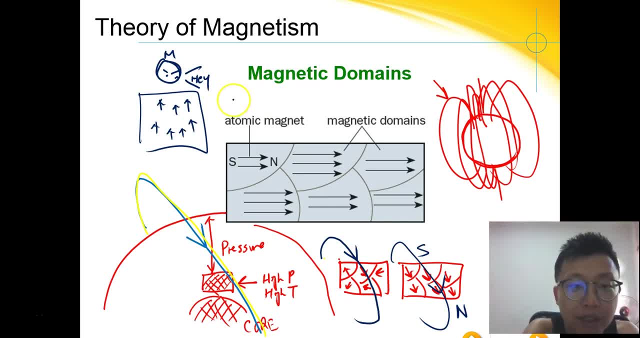 in a single direction, so magnetic domain. if you have an alignment of this domain, you can give rise to magnetism. and how would this domain align themselves? well, you have to supply heat, you have to supply pressure and, most importantly, you have to have- oh sorry, you have to have what? 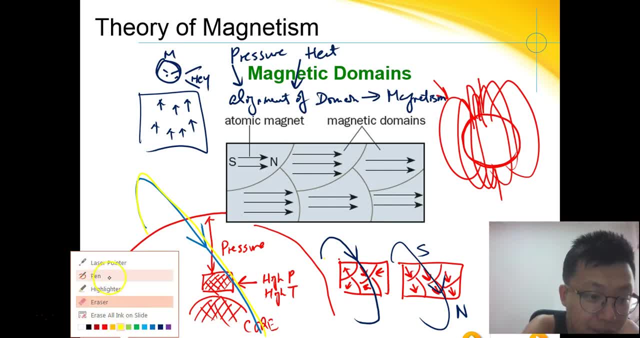 a teacher. right, you have to have a this guy, an external magnetism. you have to have a external source. you also need to have- let me get this- you also need to have a external magnetic field. okay, so how my system arises. how will you explain it? well, i have to align the domains. how do you align the domains? supply, heat. 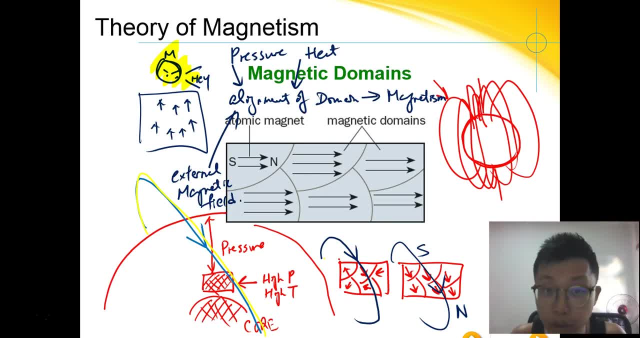 them with a external magnetic field, then you need to know, as a pure science student, why do you need heat and pressure? well, that is to give energy to the domain to align themselves. without this energy, can they move? no, they can't move. and what is the use of the external magnetic field? oh well, the external. 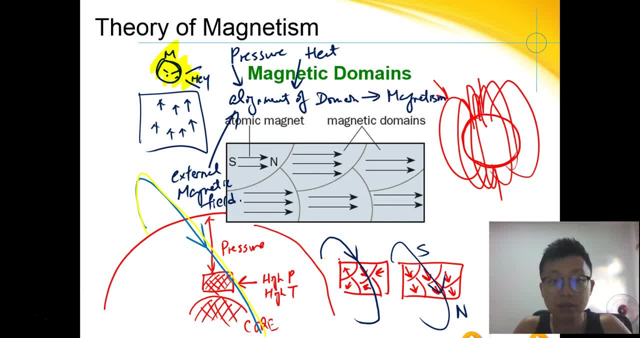 magnetic field will align the domain to a singular direction. what if there's no external magnetic field? well then, although the domain has energy to realign themselves, they do not know a line to where understand. so that is what the gist of magnetic domain.